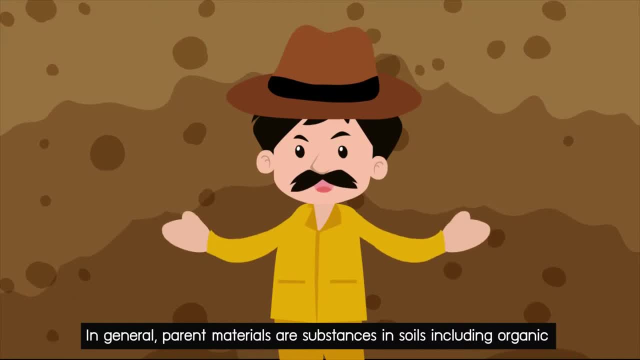 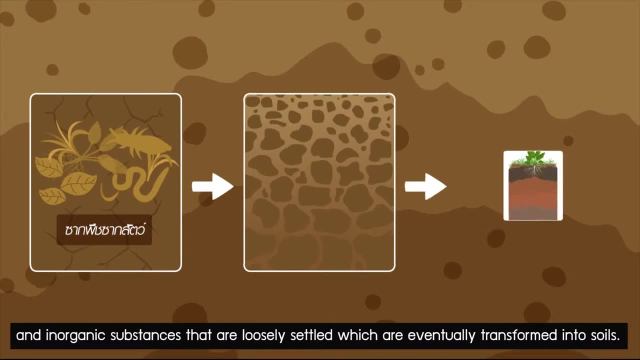 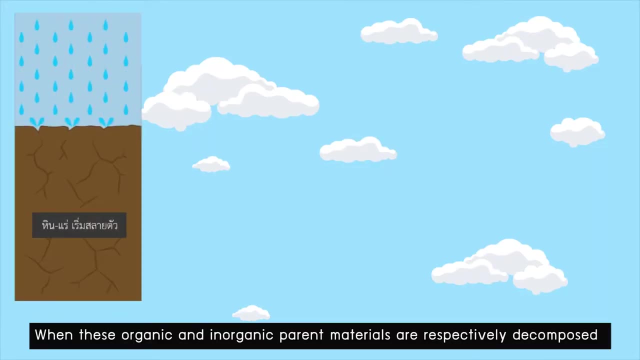 In general, parent materials are substances in soils, including organic and inorganic substances, that are loosely settled, which are eventually transformed into soils. When these organic and inorganic parent materials are respectively decomposed and weathered, they will be combined with other organic matters, thereby forming soils. 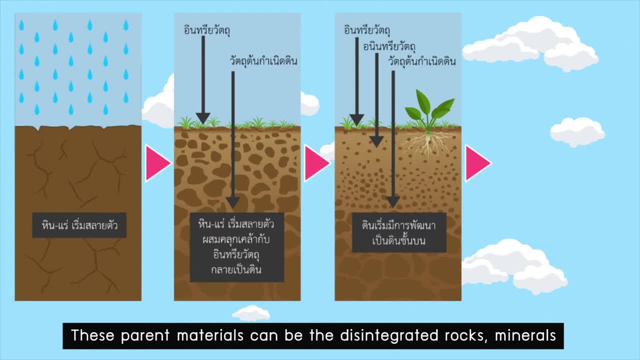 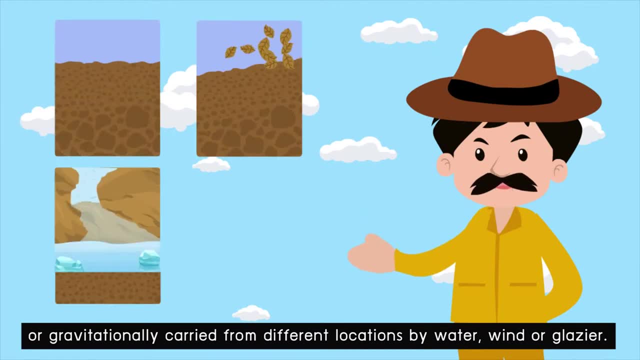 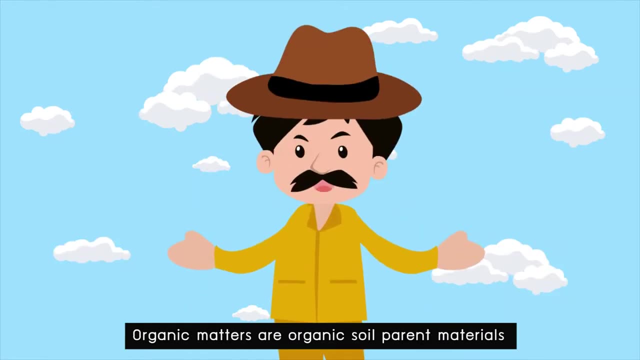 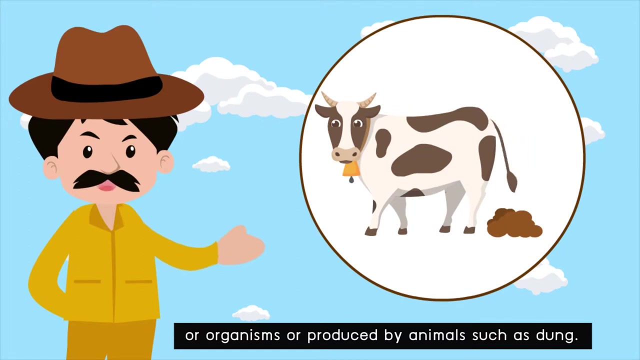 These parent materials can be the disintegrated rocks, minerals or organic matter. Organic matters in the area or gravitationally carried from different locations by water, wind and glacier. Organic matters are organic soil parent materials, which are the disintegrated remains of different plants or organisms or produced by animals such as dogs. 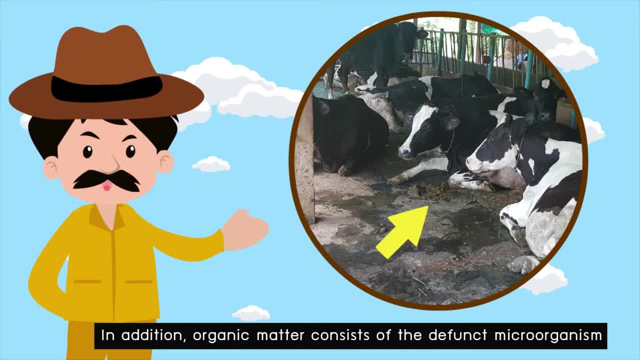 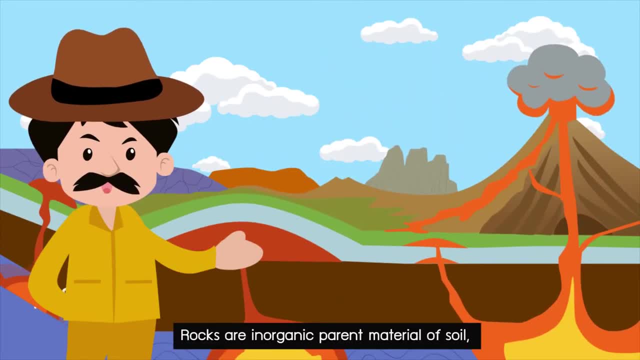 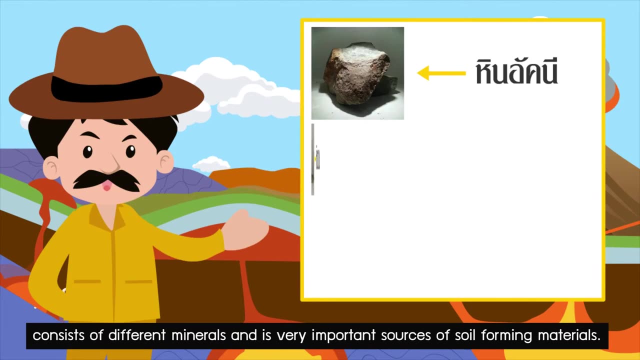 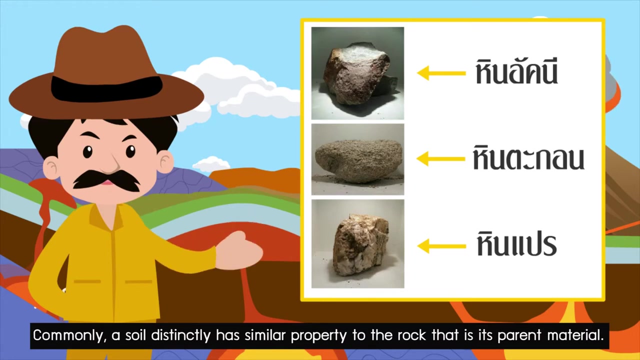 In addition, organic matter consists of the defunct microorganism or the matter produced from activities of microorganisms. Rocks are inorganic. parent material of soil consists of different minerals and is very important sources of soil forming materials. Commonly, a soil distinctly has similar property to the rock that is its parent material. 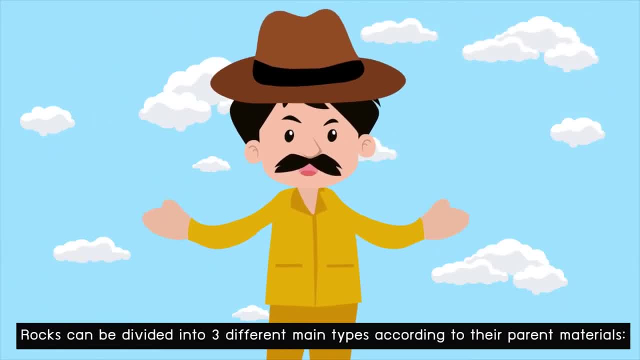 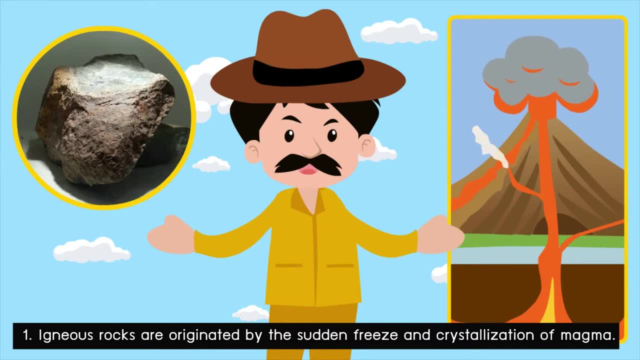 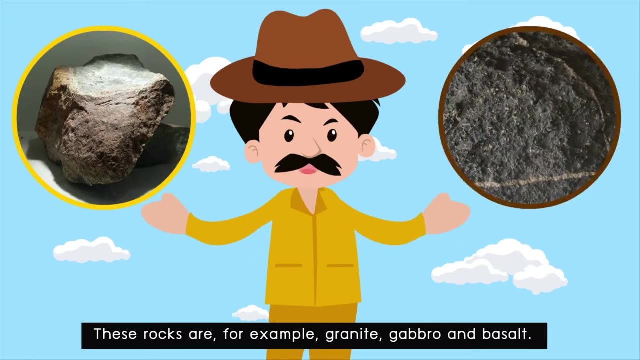 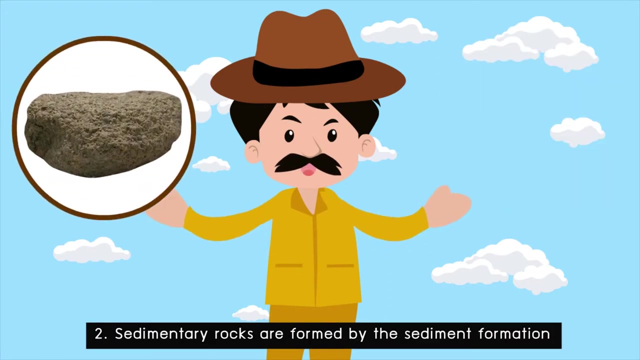 Rocks can be divided into three different main types, according to their parent materials. 1. Igneous rocks are originated by the southern trees and crystallization of magma. These rocks are, for example, granite, gabbro and basal. 2. Sedimentary rocks are formed by the sediment formation or from chemical sediment formation. 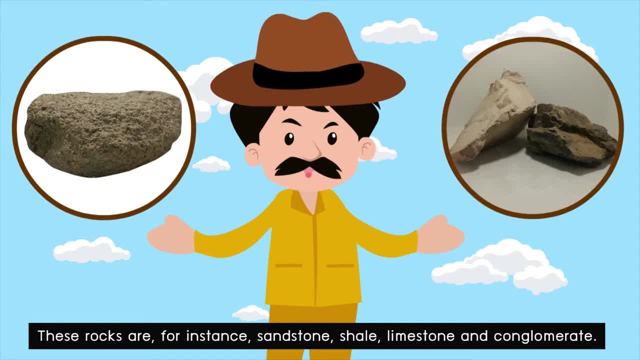 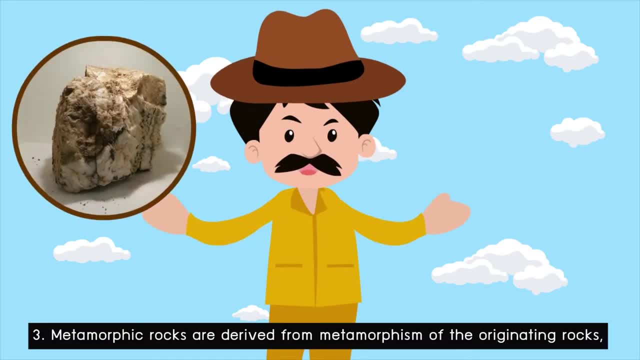 These rocks are, for instance, sandstone, shale, limestone and conglomerate 3.. Metamorphic rocks are derived from metamorphism of the originating rocks, which could be igneous rocks, sedimentary rocks and metamorphic rocks. These rocks include, for example, slate, marble and quasites. 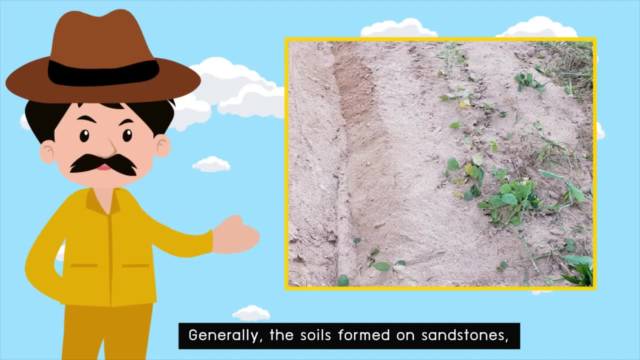 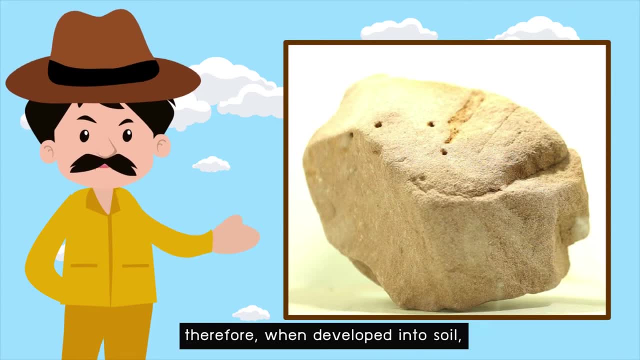 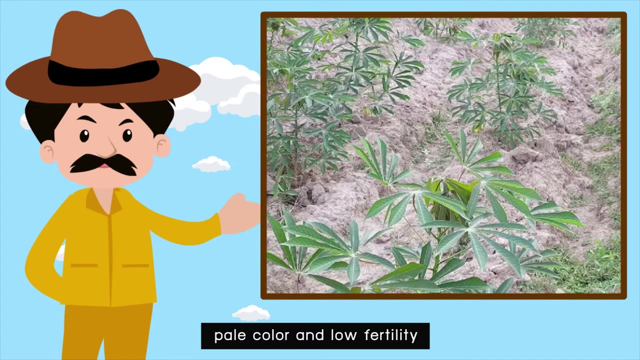 Generally, the soils formed on sandstone, Most of the component minerals, are resistant to weathering and with pale color like quartz. Therefore, when developed into soil, the texture will be forced sandy's: pale color and low fertility because of containing very small amount of nutrients for plants.